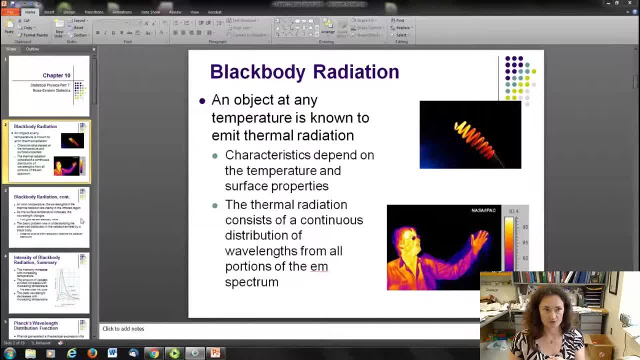 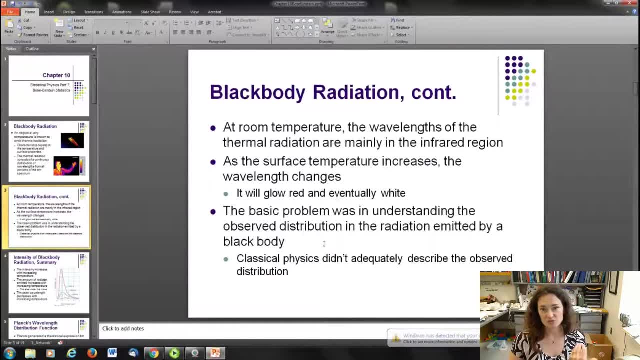 spectrum has a characteristic shape in the intensity curve. At room temperature, black body radiators emit in mostly the infrared region and then, as your surface temperature increases, the wavelength changes, going to shorter and shorter wavelengths as you increase your temperature. Classically it was difficult. 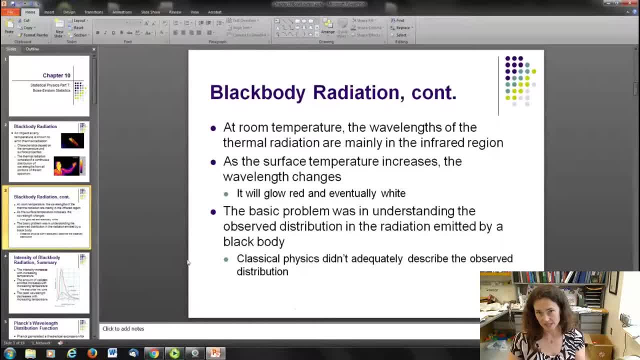 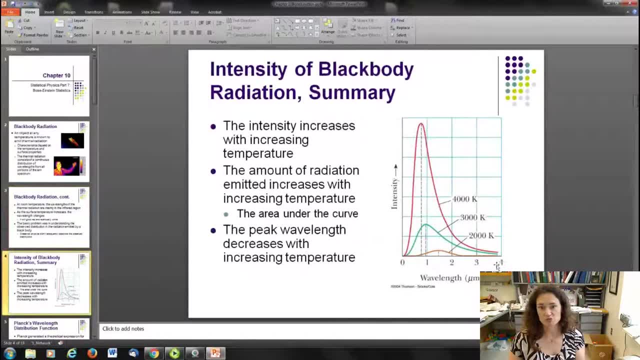 to understand why the black body curve had the shape it did. The Rayleigh-Jeans law did the best it could, but ultimately classical physics failed at describing this very characteristic intensity curve for black body radiators. Notice here that as your temperature goes, 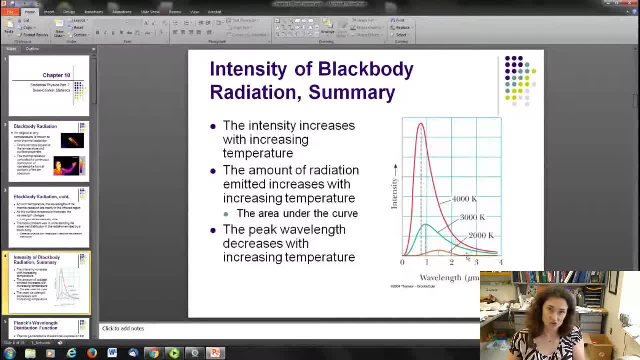 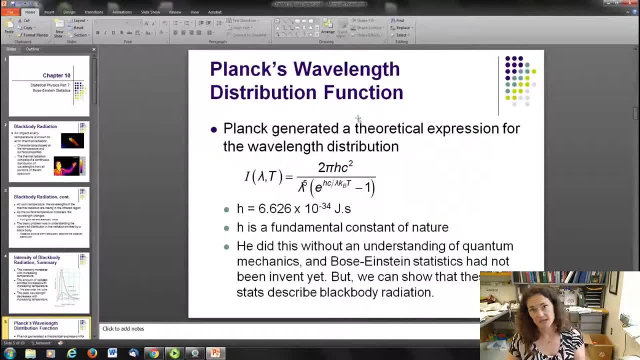 from 2,000 Kelvin to 4,000 Kelvin. the wavelength gets shorter and shorter, moving there to the left. What Max Planck did is he fit the curves, and then it came up with a theory that best described why the curves act the way they do. To describe the theory he had, 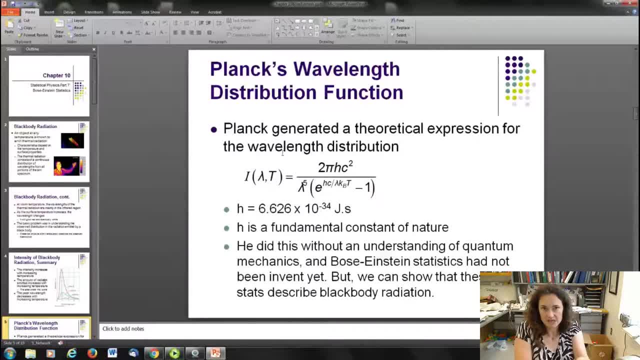 to assume that a solid was a collection of atoms kind of connected to one another by these little springs, And the springs only vibrated at very specific quantized frequencies. Okay, So this was a new idea and helped lead us into the quantum mechanics that we know. 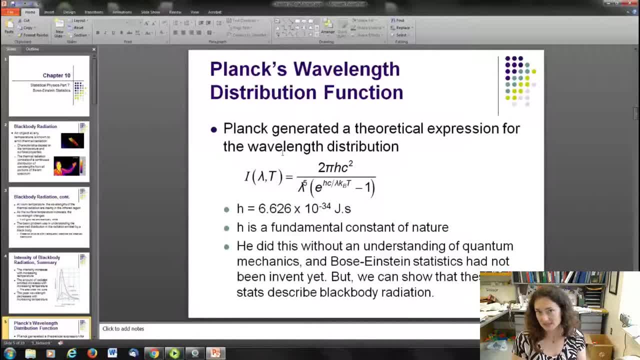 and love today. But it's worth emphasizing that Planck did this. he derived this expression for a black body radiator's intensity curve without any other kind of information. So this is a very interesting theory, Knowing anything about quantum mechanics or knowing anything about Bose-Einstein statistics. 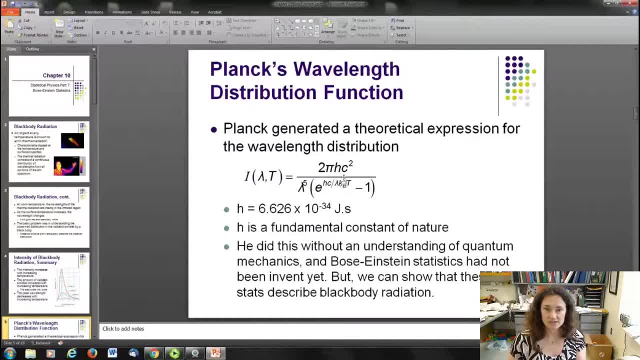 which weren't developed until much later. So here's our intensity curve. The intensity, which is a function here of the wavelength and the temperature, is equal to 2 pi hc squared lambda to the fifth over lambda to the fifth, e to the hc over lambda, kt minus 1.. Okay, 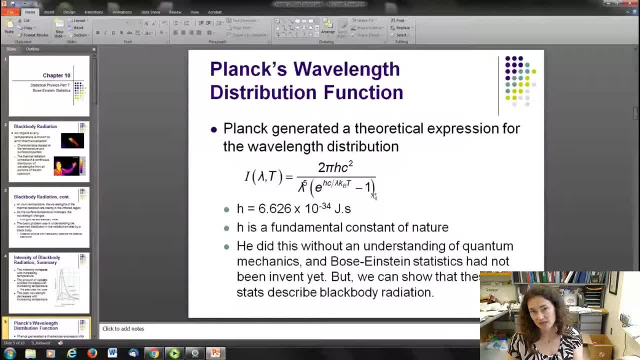 Now that e to the hc over lambda kt minus 1 bit. that should look like. here's the energy of our photon hc over lambda kt minus 1.. Okay, Okay, So that's actually e to the e over kt minus 1.. Okay, And that should look somewhat familiar. 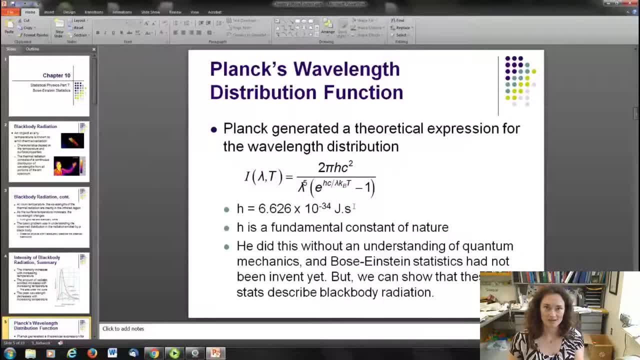 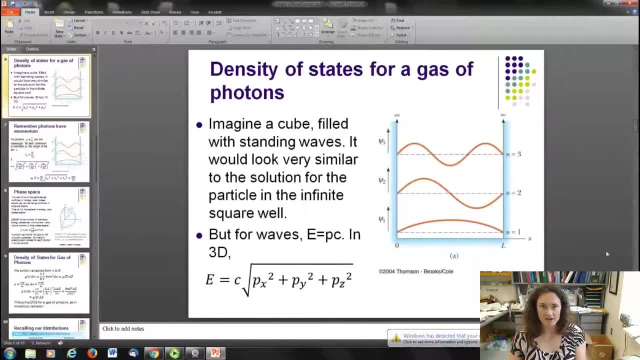 after the last two lectures, because that's part of our Bose-Einstein statistics distribution function. Okay, So spoiler alert, All right Now. first, in order to describe Bose-Einstein statistic for black body radiators, we have to develop an expression for a density of states. We can't use the one for a gas. 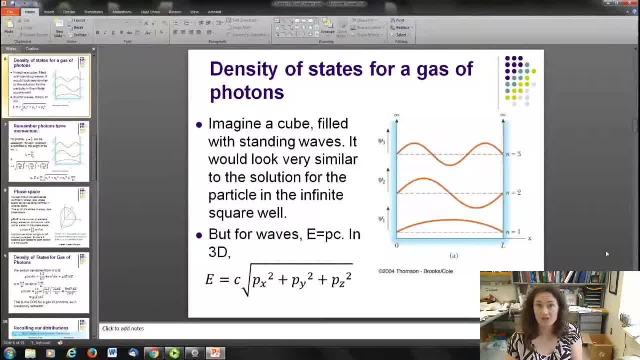 of particles that we've been using for the last several lectures, Because for black body statistics, you're actually generating a gas of photons. This is the light that gets emitted by a black body radiator, So that's not a particle per se, It's a photon, And they have different kinds of expressions that govern them than 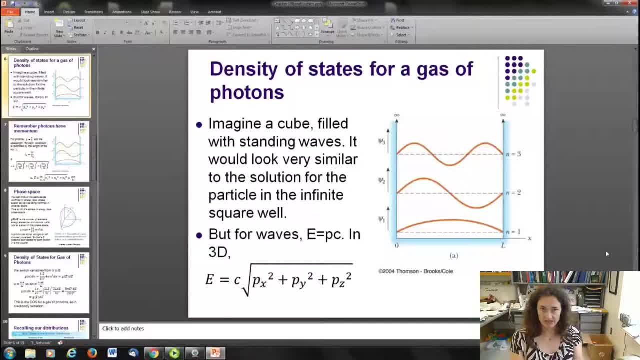 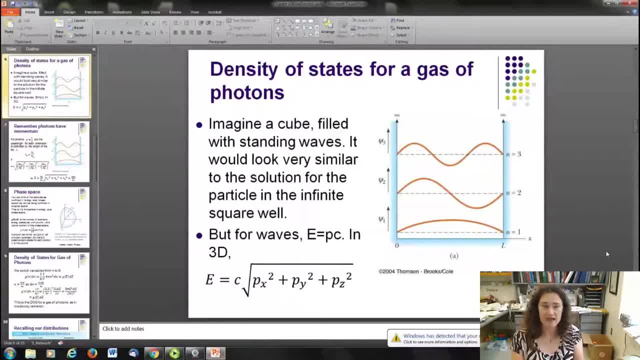 of a black body. So we're going to do that inside the cube. Wavelengths of light can exist in the cube, But they have to form standing waves because they interfere with one another, And all other waves that don't have the wavelengths that form standing waves are going to cancel. 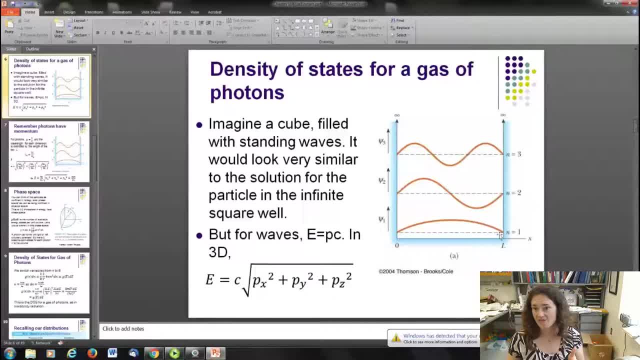 out. So the standing waves you're going to form a half wavelength kind of value. So in your ground state you'll have one half wavelength, In your first excited state two half wavelengths, and so on and so forth going up from there. Okay, 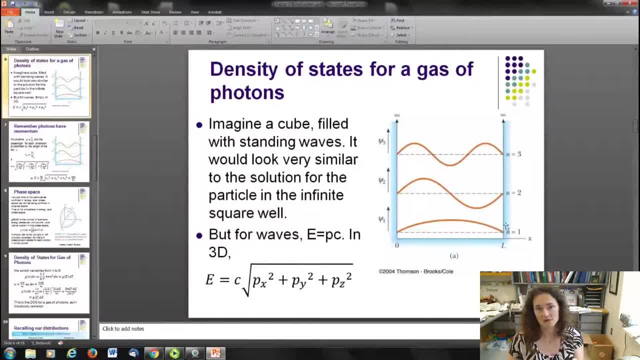 Now the wavelengths that form dictate what the momentum of the light is. Remember we're, as we covered pretty extensively in modern one. light has momentum. okay, now for waves. the energy of the wave is equal to pc. this is hc over lambda. e is equal to hc over lambda, where p is the momentum of the wave. 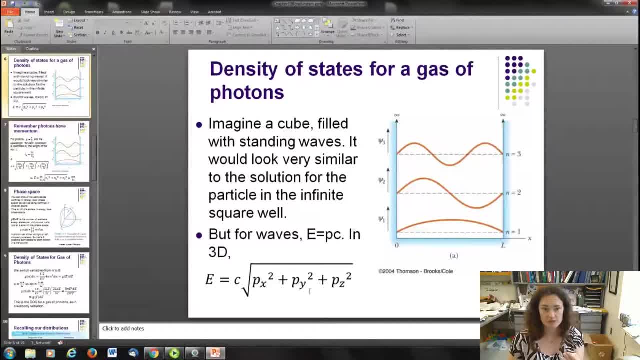 which is h over lambda. now we have a 3d problem. so we've got momenta in the x, y and z directions. so our total momentum, p, is the square root of the sum of the squares of the momenta in the x, y and z directions. 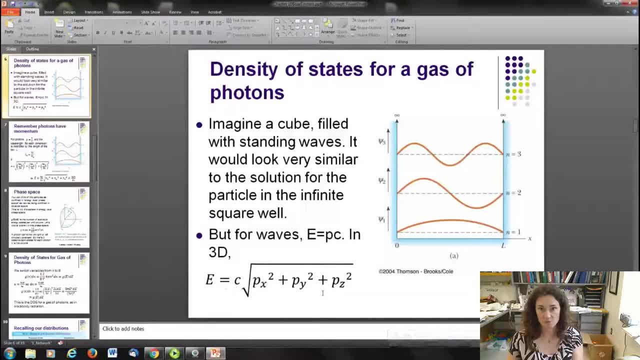 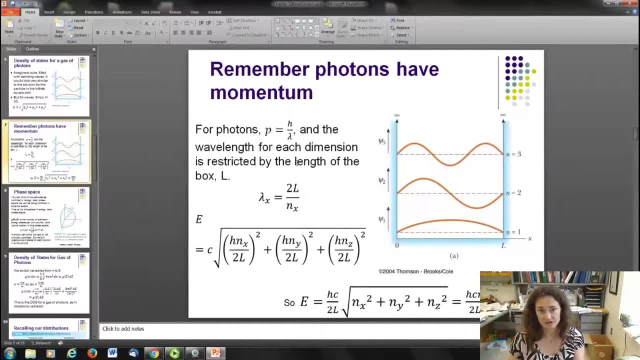 so we have: e is equal to c times the square root of p x squared plus p y squared plus p z squared. so remembering that p is equal to h over lambda and the wavelength for each dimension is restricted by the length of the box, if you look here you've got one half wavelength confined in. 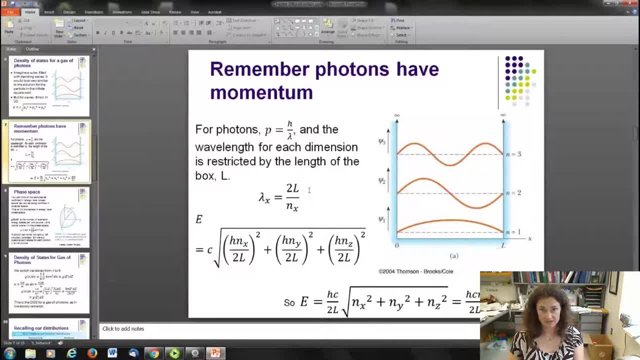 this box of side l. so that means that the wavelengths are actually going to be equal to 2l over n for each direction: x, y and z. okay, in other words, if it's in the ground state and n equal to 1, then the total wavelength here is 2l. and then for the first excited state, 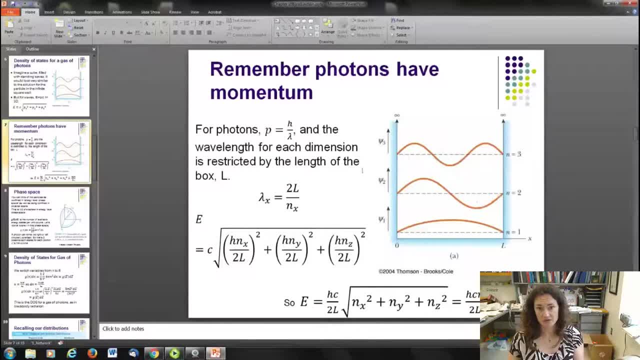 you've got one full wavelength confined in the box and its wavelength would be l over 2. hope you understand that and see it, but if you don't, go ahead and pause the video and take a second to make sure to really take that in, okay, now plugging in for lambda equaling. 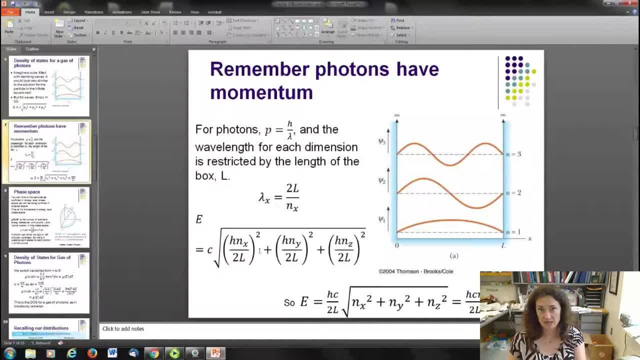 h over p. plugging in there and finding and solving for p in each dimension here. plugging those values in, you get. e is equal to c times the square root of h, n over 2l squared. and then summing that up for the x, y and z directions, if i pull, 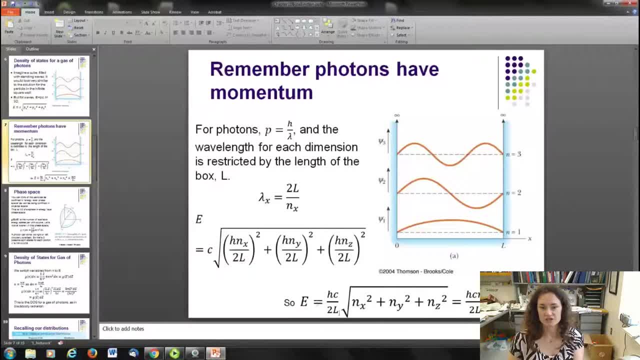 common factors out then i have: e is equal to h, c over 2l times the square root of the sum of the squares for the quantum numbers in the x, y and z directions: n x squared plus n y squared plus n z squared. if we use the idea that we developed in a previous lecture, 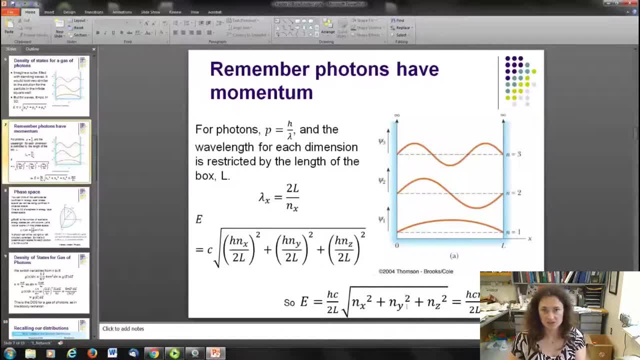 that our quantum number n is equal to the square root of the n- x squared plus n y squared plus n z squared. then we can solve and find that e is equal to n- y squared plus n z squared, equal to h, c, n over 2l. okay, so that's our energy expression and it's different from: 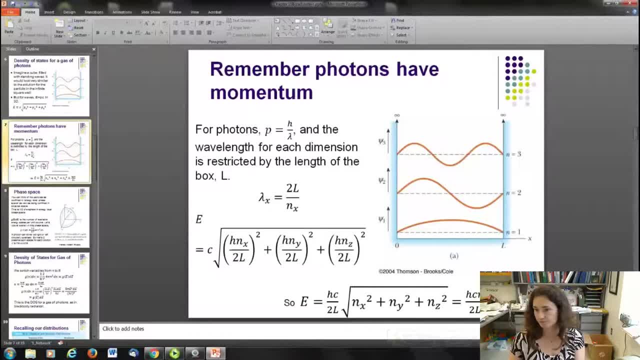 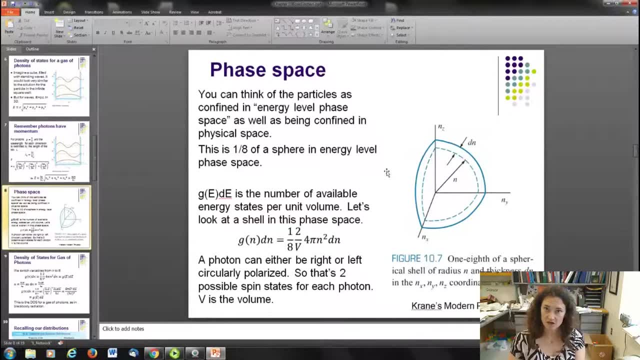 the energy expression that we derived for the gas particles. but we're going to use the same kind of idea, in that we're going to put this in phase space, okay, and the phase space here is going to be our energy level space, and then we're going to switch that over to. 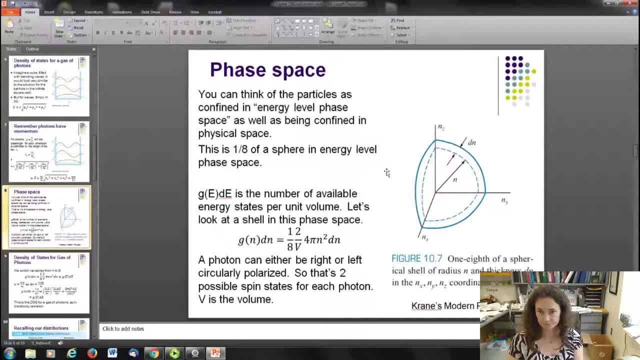 energy with a change of variable in just a little bit. remember that you can't have any negative values for your energy levels. they have to start at one and go up, and so that means that only one quadrant of the little sphere that's formed in phase space is going to be useful to us, so we're going to have one eighth of a sphere in energy. 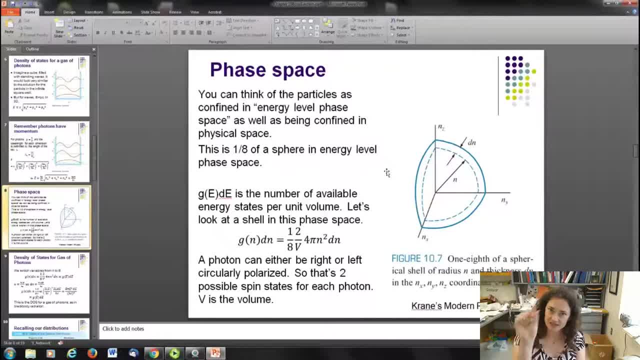 level, phase space, and we're just looking at a little slice of that sphere because we want to know what the density of states is right. so the density of states is going to be this factor of one eighth and then times one over the volume, because the density of states is 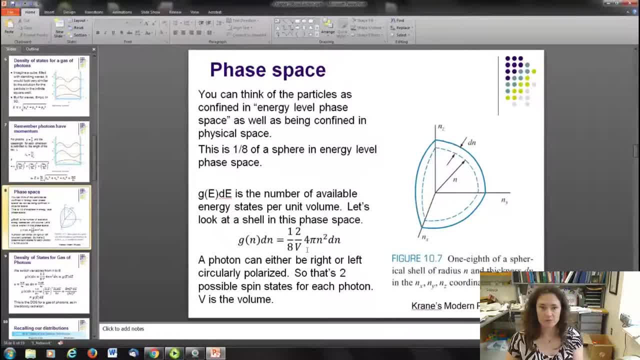 energy per unit volume. so the volume is important there. and then we have our four pi? n squared. that's the area of our sphere in phase space. and then to get the volume we multiply that times d n, which would be the thickness of our spherical shell. now, this factor of two 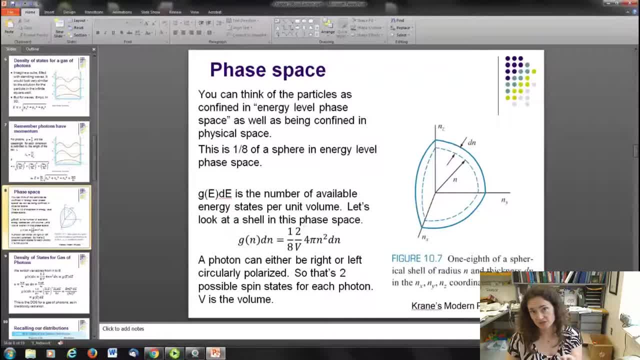 here is because there's two possible values for the spin of a photon. remember, in the gas of particles we had two s plus one to account for the multiplicity of the spin states. but for a photon there's only two choices: it's either right, circularly polarized, or left. 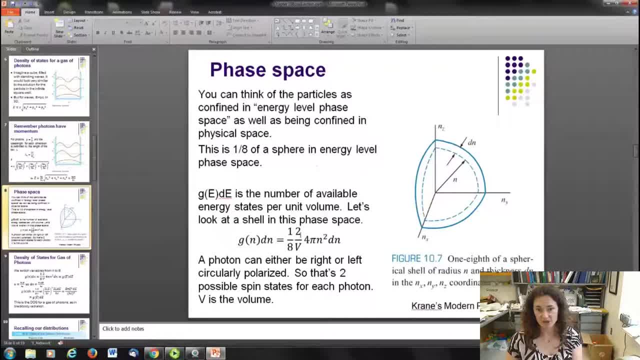 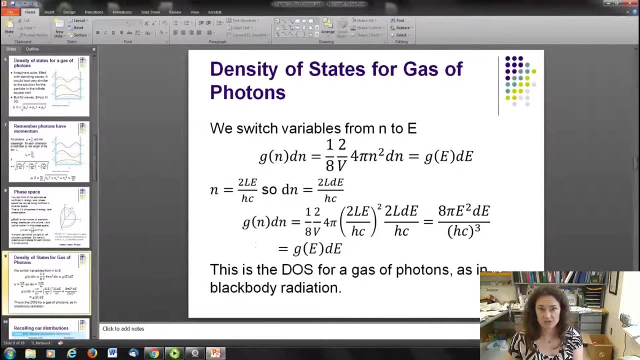 circular, circularly polarized, and so that's that value of two that we put in right there. so this is our expression for the density of states in our, in terms of our, energy level, n. now, if we want to switch that over, we change variables from n to energy just using the expressions relating the energy and the energy level. that. 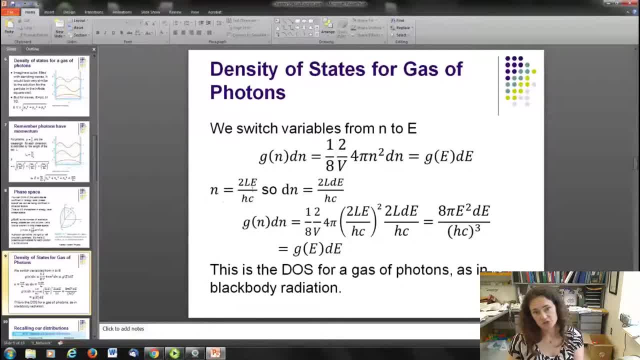 we derived earlier rearranging that n is equal to two l e over h c and then d n is equal to two l d e over h c. if i plug in for that value of n and d n into my expression for my density of states, then after a little bit of algebra i get eight pi e squared, d e over h c cubed, and that's. 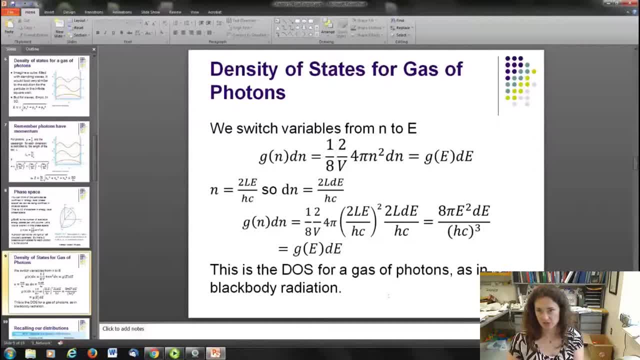 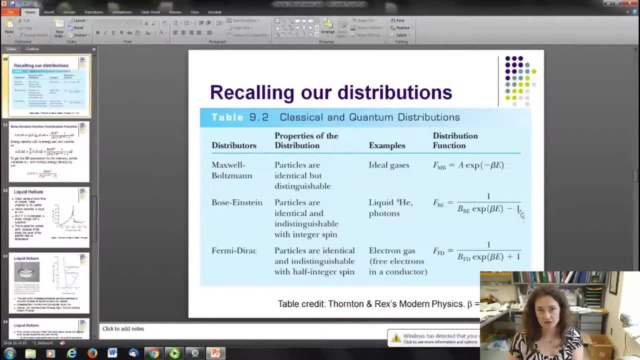 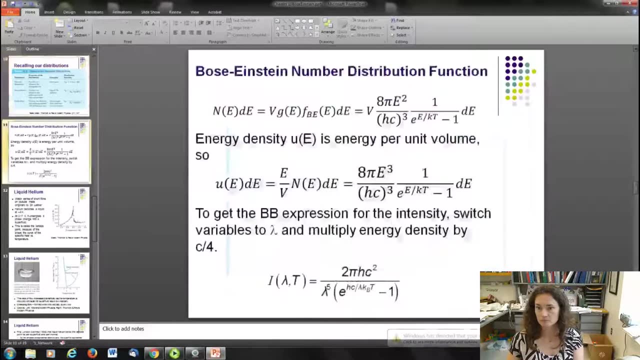 our density of states for a gas of photons, like a black body radiation type thing. now, recalling our distribution functions, here's our Bose-Einstein one here for integer spin. remember that photons can be considered to be particles of integer spin. alright, so what we're going to do is to get our numerical distribution function. we're going to multiply. 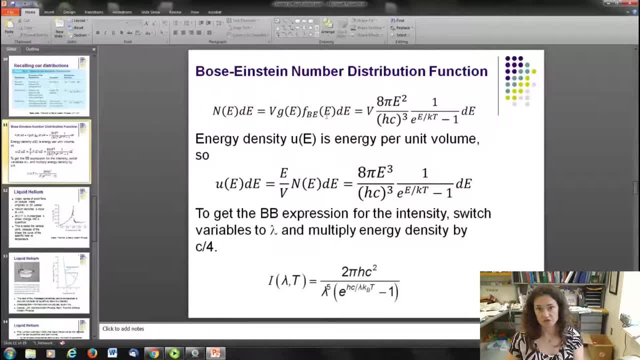 our density of states times that distribution function for Bose-Einstein statistics, we get then the eight pi e squared over h, c, cubed one over e to the e over k, t minus one d e. so that's our numerical density of states. now, if we want to relate that back to Planck's, 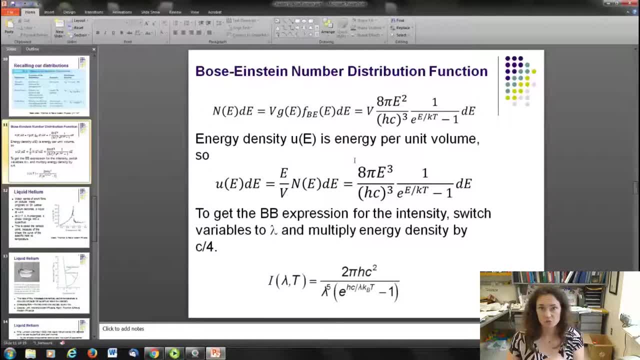 expression for the intensity, then we need to switch over and not look at the numerical density of states, the number of states, but we would need to look at the intensity of the emitted radiation. in order to do that, it's first best to switch over to the energy density, because you can. 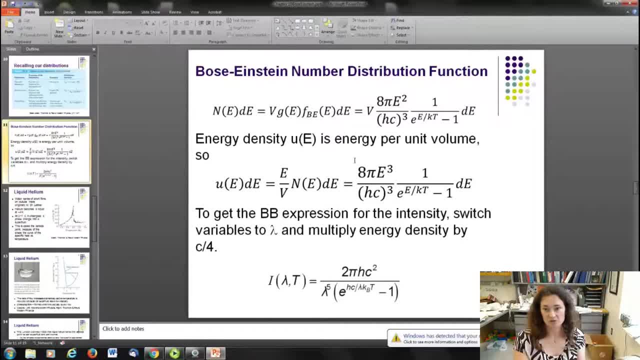 relate the energy density to the intensity by multiplying simply by c over four. so if we switch over to the energy density, that's the energy per unit volume times the numerical distribution function, and then we have eight pi, e cubed over h, c cubed, one over e to the 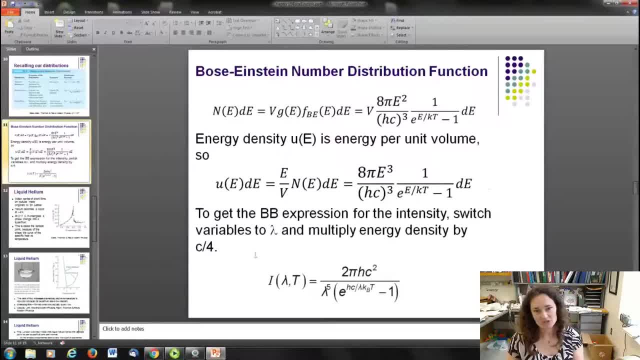 e over k, t minus one, d e, okay, and then we just multiply that by c over four and we integrate it, and there's our expression for our intensity. okay, so way to go. Planck, thinking of all of this stuff many, many years before quantum mechanics and before Bose-Einstein statistics. 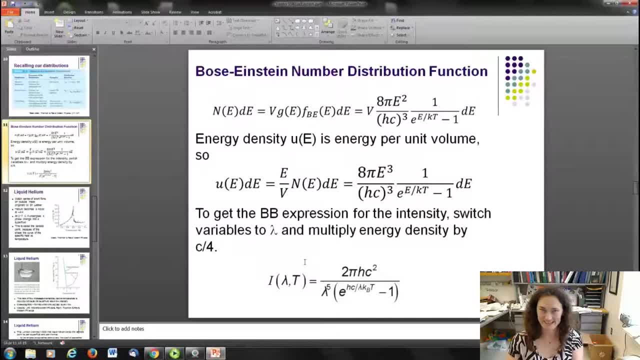 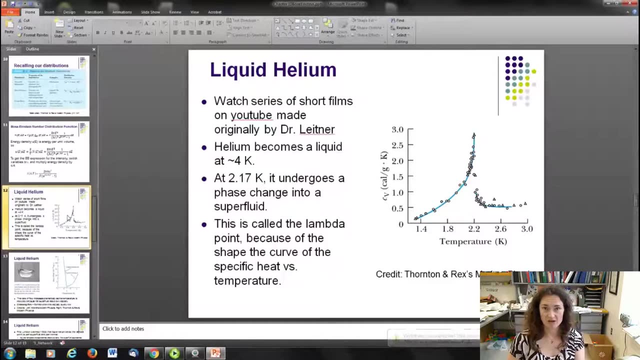 but way to go, Bose-Einstein, for realizing that you have this set of statistics that describes this, and much more. as it turns out, now there's some really fun videos that I have posted. underneath this video, it's a series of YouTube films made originally by Dr O'Barr. 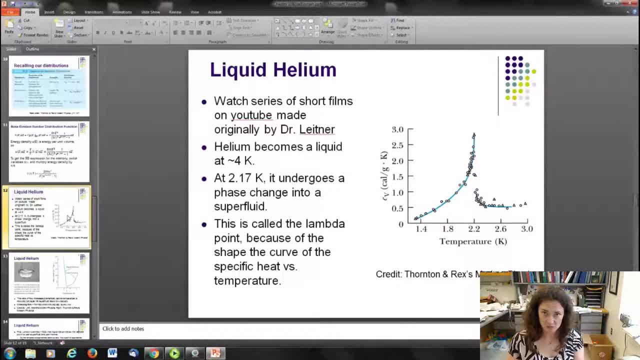 Leitner in the 1960s, and he explores and explains some of the really interesting properties of liquid helium. now, helium is a noble gas, so it interacts very weakly with itself, all right, which explains, or helps explain, why it doesn't even become a liquid until such. 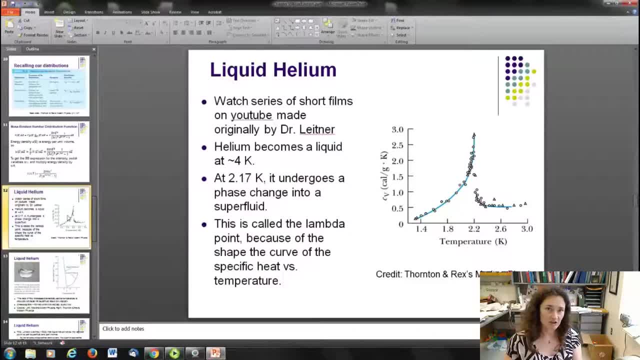 a low, low temperature, about four kelvin. remember that all the noble gases become liquids at low temperatures. but helium goes even lower than the others because it's so lightweight, amongst other reasons. now, if you cool liquid helium down even further, towards what's called the critical point or the lambda point, it'll start to boil very violently as 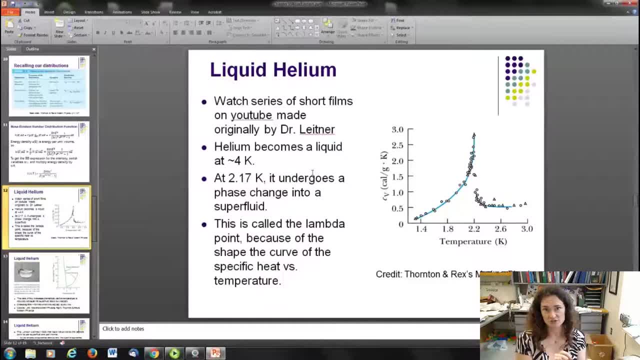 it gets close to that lambda point and then once it reaches 2.17 kelvin, that critical temperature, it goes perfectly still and then you know that's actually achieved a phase change and become what's known as a super fluid. all right, it's called the lambda point. 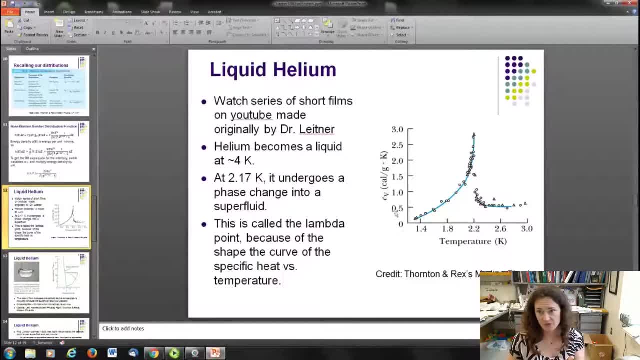 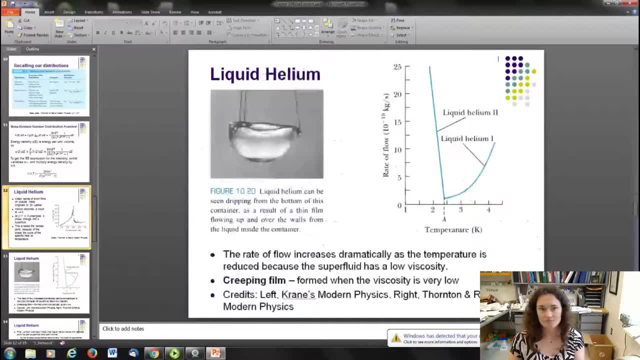 because if you measure the heat capacity and clock the heat capacity versus the temperature of helium, it actually makes a really cool lambda shape that you see here on this plot. so liquid helium, attir below the lambda point, exhibits interesting properties on super fluids all do this. one of those really interesting properties is that it has a very, very close 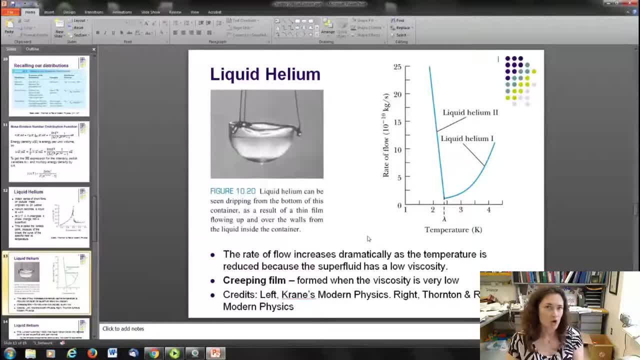 zero viscosity, basically no viscosity. remember that viscosity isn't a liquids resistance to flow. So if you have a viscosity of zero, then the liquid basically has no resistance to flow at all. That means that the film can do really cool things like creep up over the edges of the container. 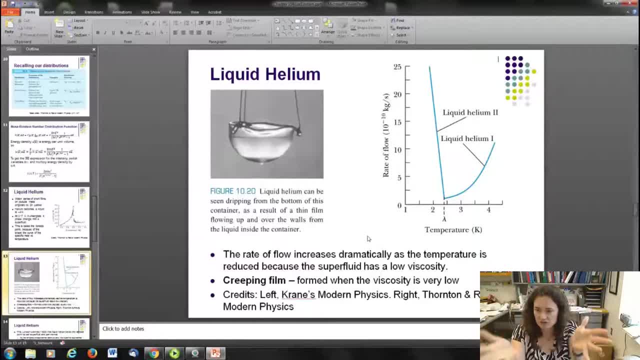 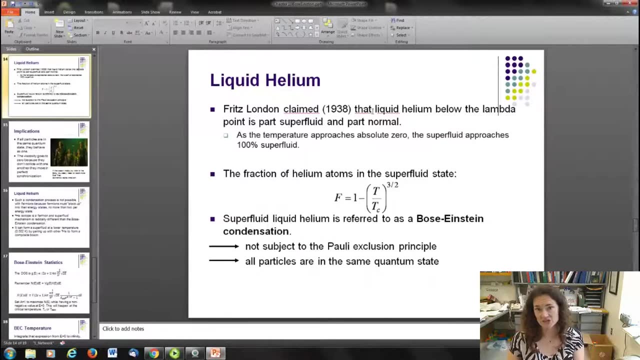 It forms a very thin film and it creeps up over the edges and then drips down the bottom. Some of Dr Leitner's videos show this very, very low viscosity feature of liquid helium. Now Fritz London, in a paper in 1938, actually said that liquid helium below the lambda point is part superfluid and part normal. 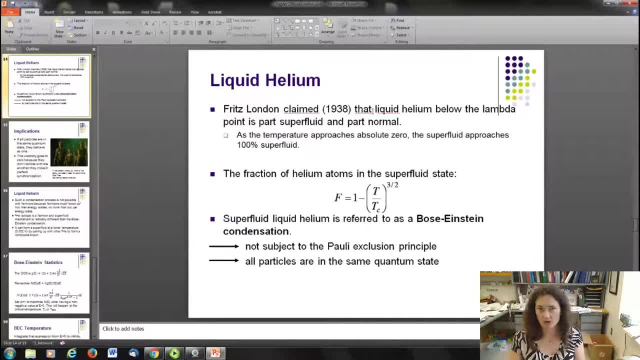 And that as your temperature gets lower and lower and lower and lower, which they weren't really able to do very well in 1938, so this is a pretty incredible prediction for him to make, actually, that the fraction of helium in that superfluid state changes as the expression 1 minus T over Tc. 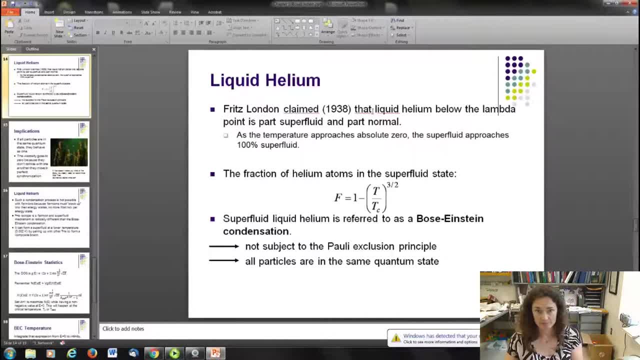 where Tc is the critical temperature. Tc is the critical temperature raised to the three-halves power, So superfluid liquid helium- the part of liquid helium that's in the superfluid state- is referred to as a Bose-Einstein condensate. 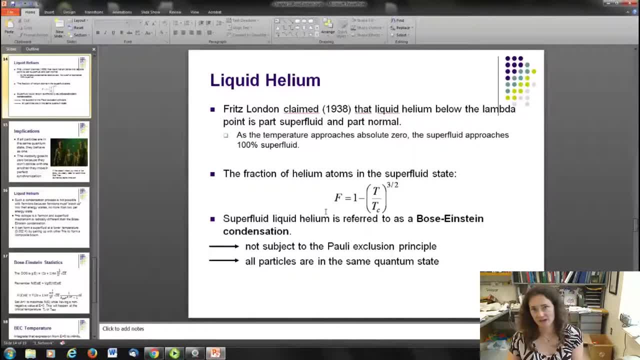 Okay, you may have heard this expression in physics and kind of wondered what the heck they were talking about. All right, so Bose-Einstein condensates are all particles that are in the same quantum state. Bosons can do this because they have integer spin and are not subjected to the Pauli exclusion principle. 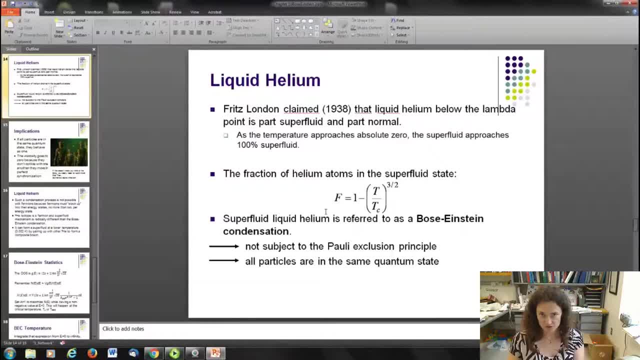 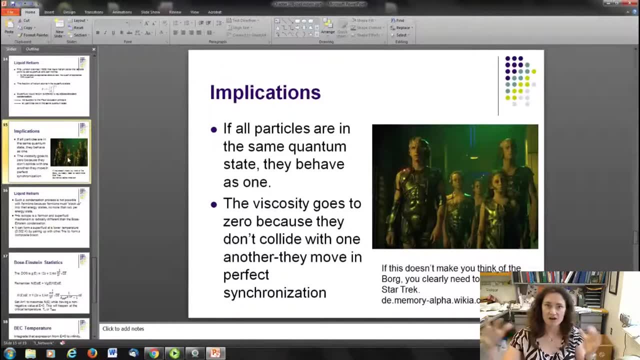 So what happens in a Bose-Einstein condensate is: all the particles fall into the same quantum state, which means basically, if they're all in the same quantum state, they have perfect knowledge of every system, everything in the system. They all know where each other is. 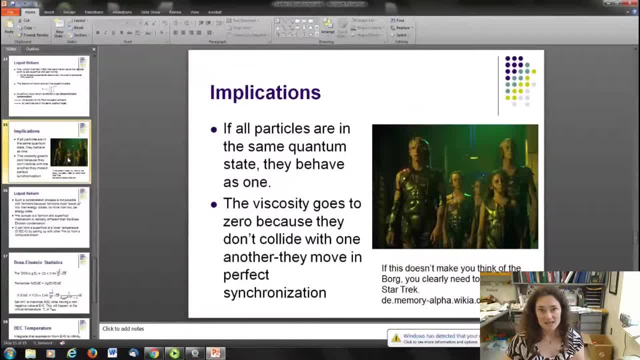 They're behaving basically as one, So the viscosity can actually go to zero because the particles don't collide with one another anymore. They're moving in perfect synchronization together, and that's one of the reasons that superfluids do what they do regarding the viscosity. 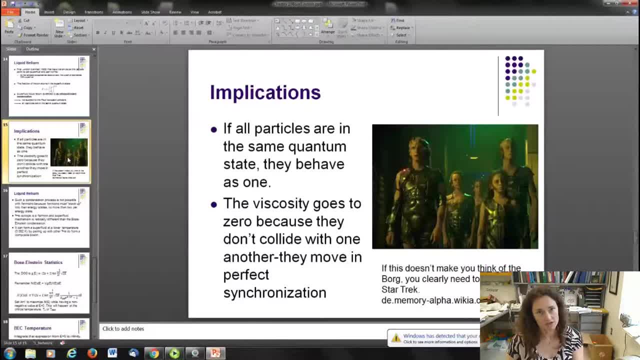 Now, if this doesn't make you think of the Borg, you really need to watch a little bit more sci-fi, a little more Star Trek. You need to get into the nerdiness that you have joined by becoming a physics major. It's actually pretty enjoyable. 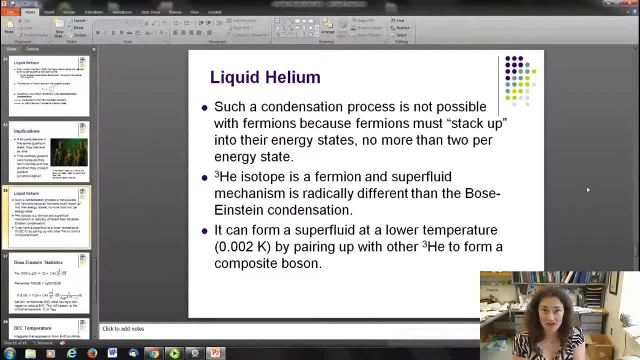